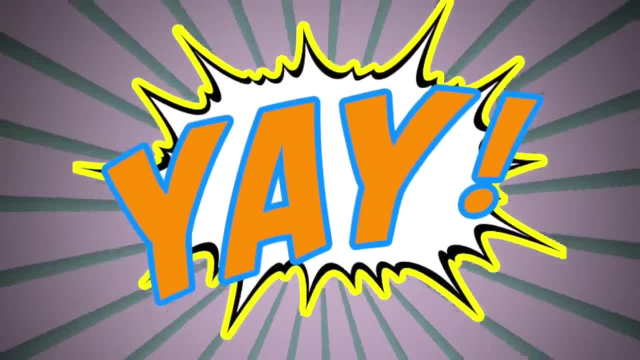 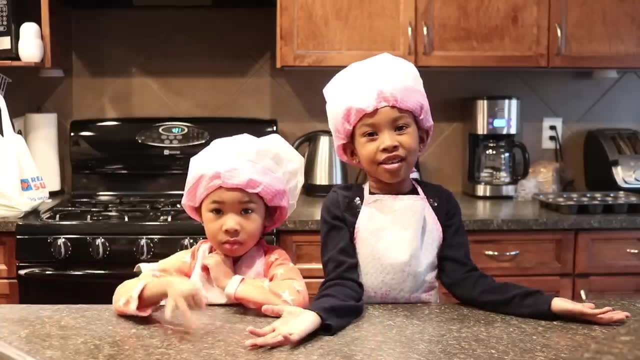 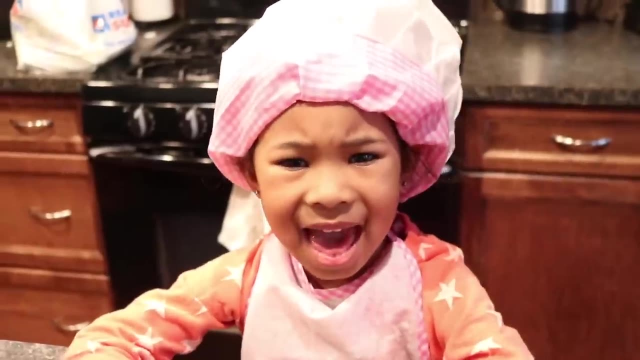 I have the perfect easy recipe for you girls to do: Yay. So, Daddy, what's the easy recipe? what you got for us, It's banana bread. Mmm, yummy, I love banana bread, Banana bread, Put a banana and bread together. 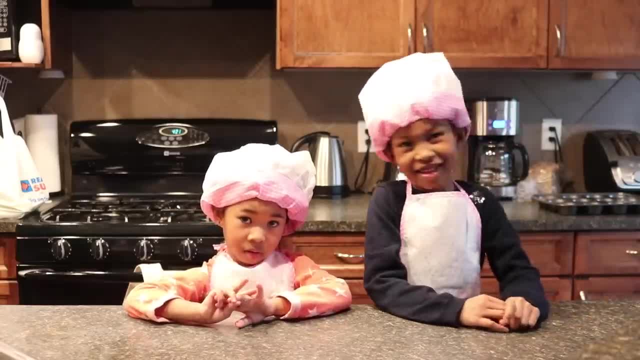 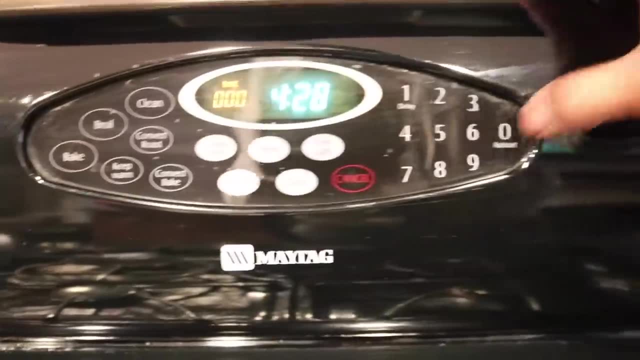 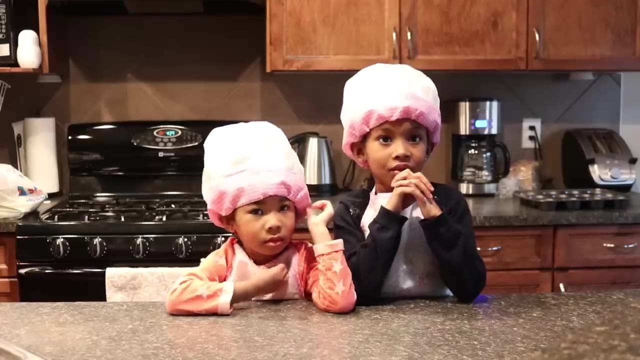 It's not just a separate banana and bread and you put it together. no, There's a lot more steps to that, but it's pretty simple. Let's just get started. Okay, We better stay awake, okay. Okay, girls, since you said you wanted to do it by yourself, 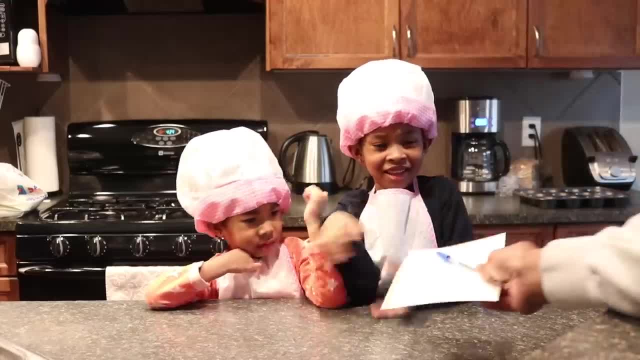 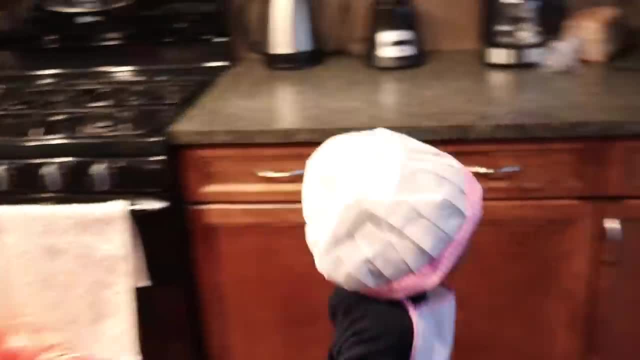 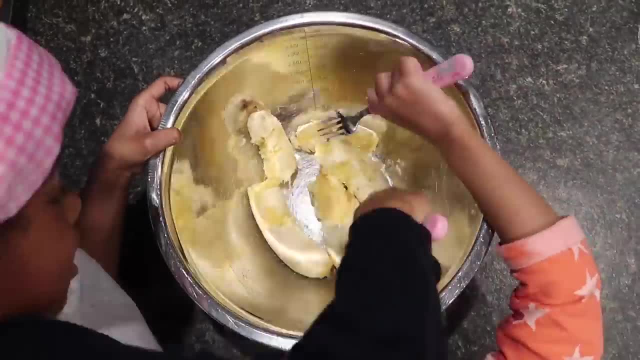 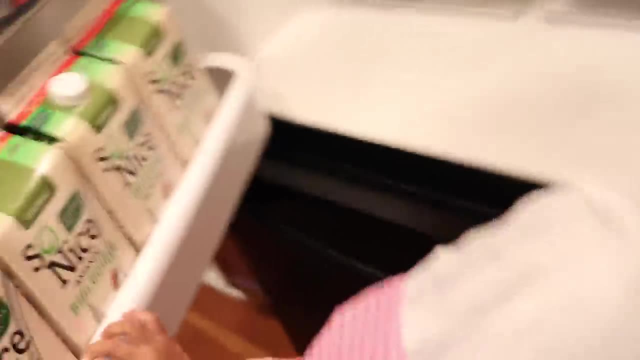 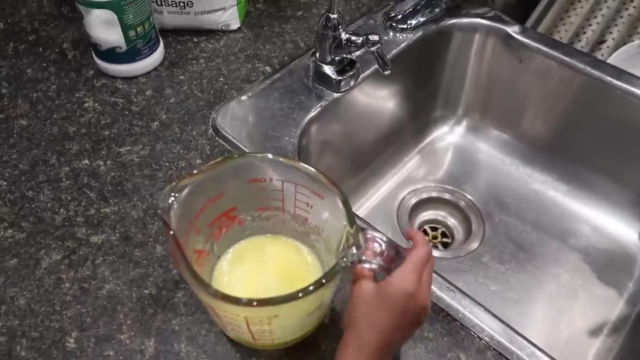 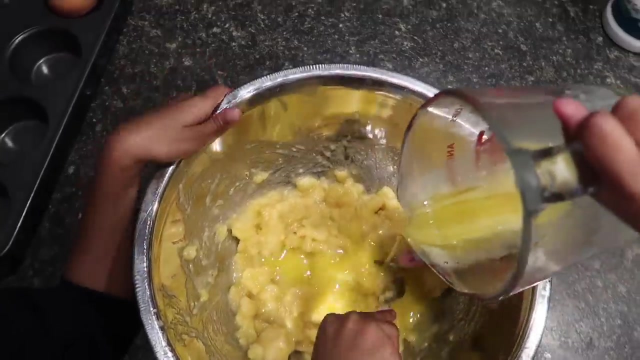 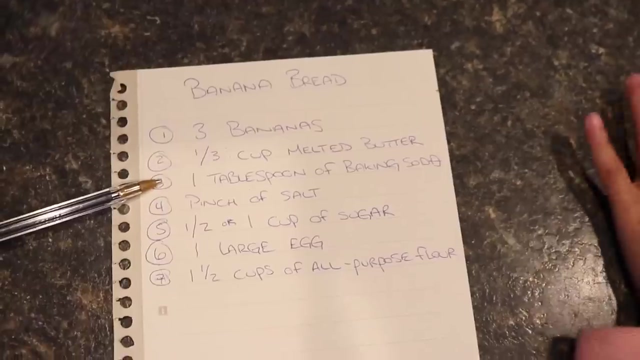 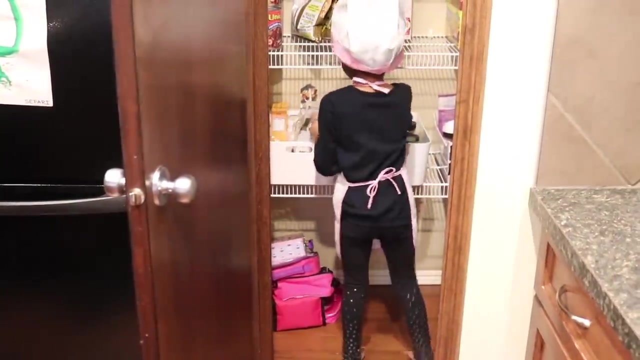 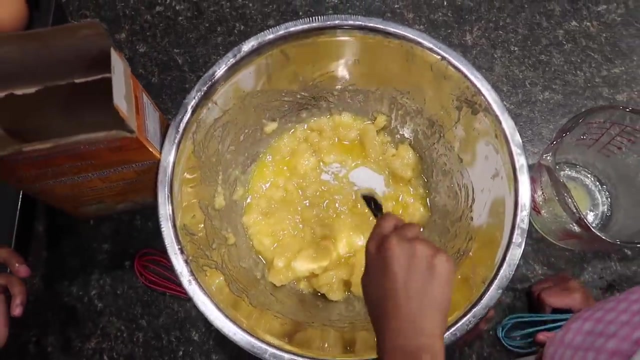 acha. A quarter cup of melted butter. Butter, butter, butter, Butter, butter, butter. One or two, You want to fold it with that butter. One tablespoon of baking soda, Teaspoon of baking soda. Can I mix too? 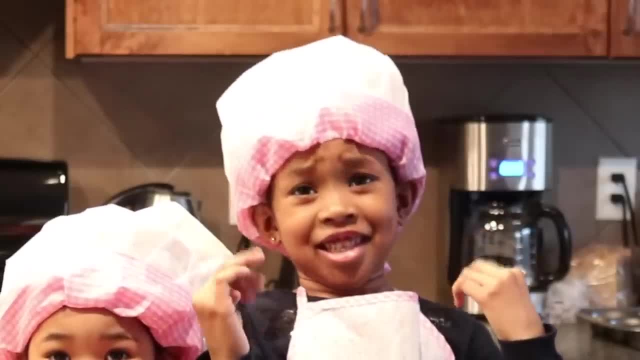 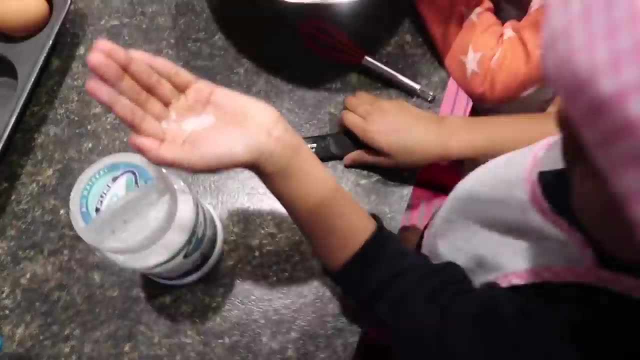 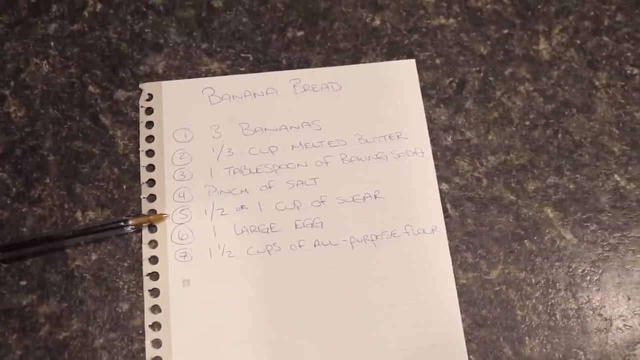 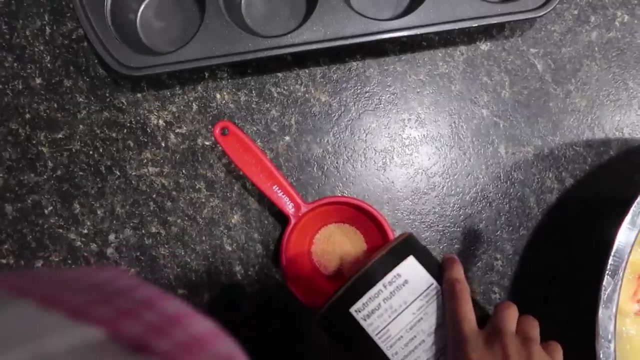 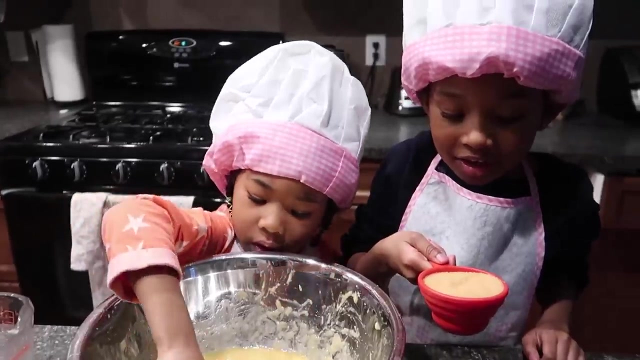 A pinch of salt, Salt, That's enough. A half or a full cup of sugar, Sugar, Sugar, sugar, sugar, Sugar, sugar. Got some sugar. That's a lot of sugar. Oh no, no, no, no, no, no. 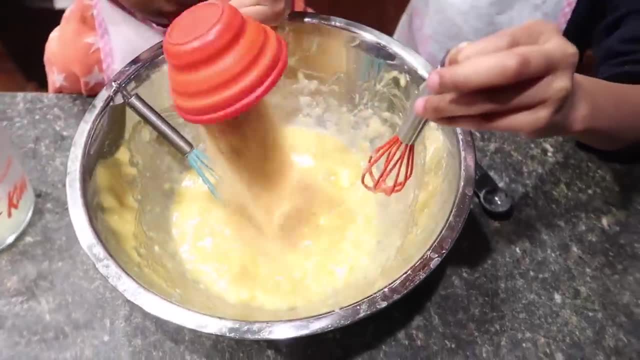 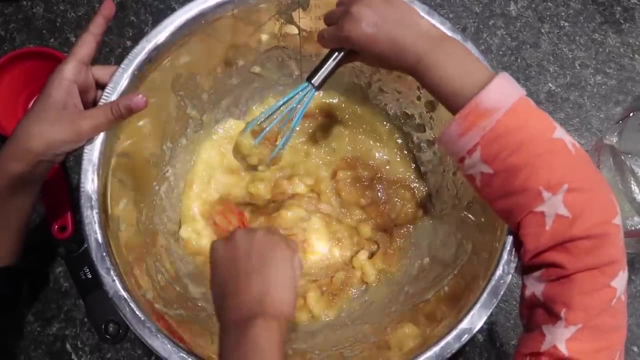 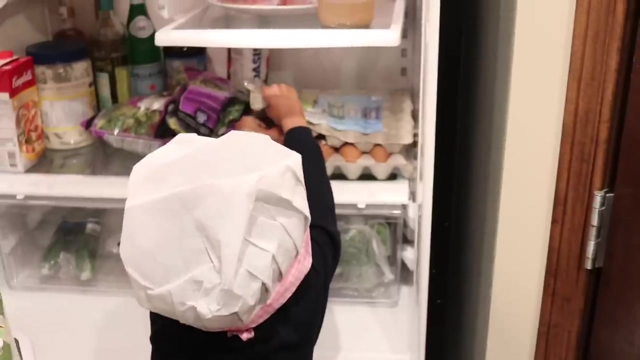 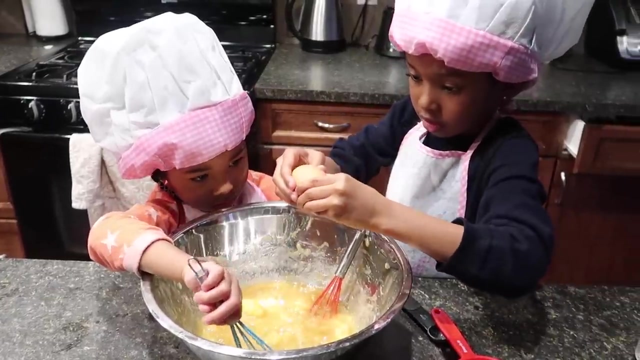 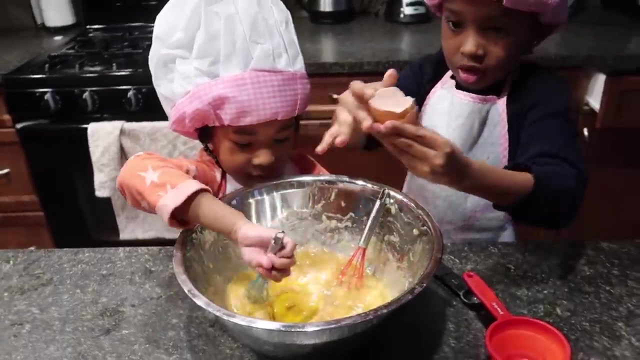 That's okay, Let's dump it in. Oops, Mix, Mixity, baxity, bax. Let's mix it. Mix One blocked egg Egg. I'm so scared, I'm so scared, I'm so scared, It's yucky. 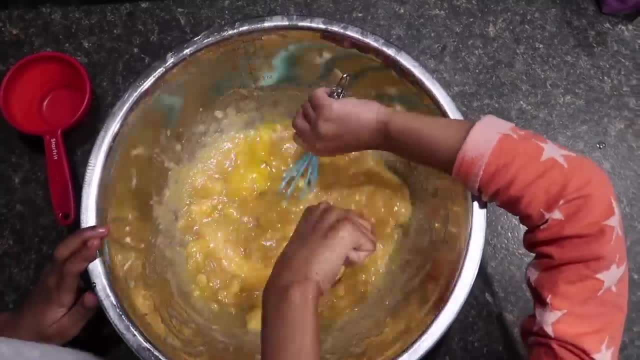 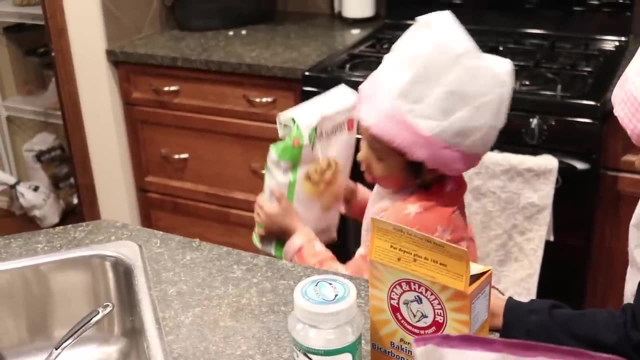 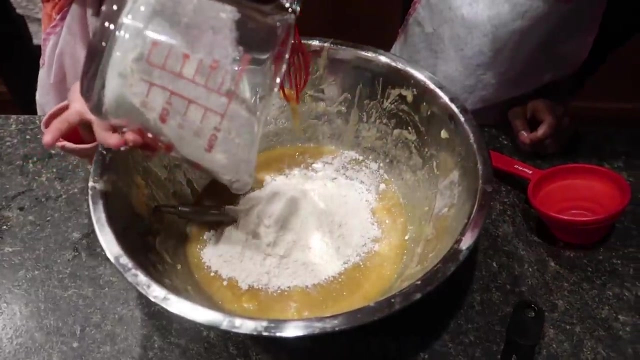 Uh-oh, Now we have to mix the egg up. One and a half cups of flour, Get it up there. That was heavy, Oh your spoon. Now, since the dough's all done, let's get our baking cups all ready. 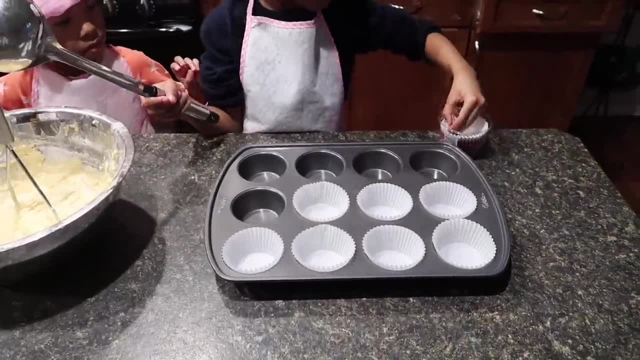 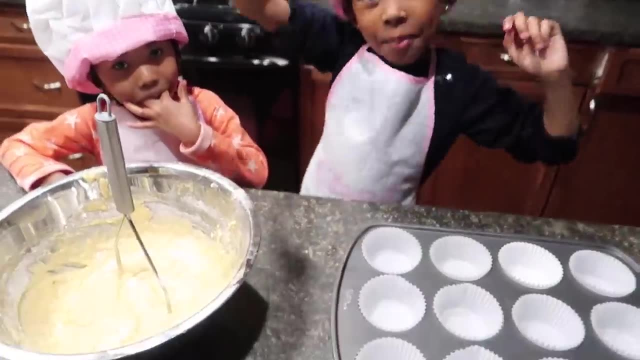 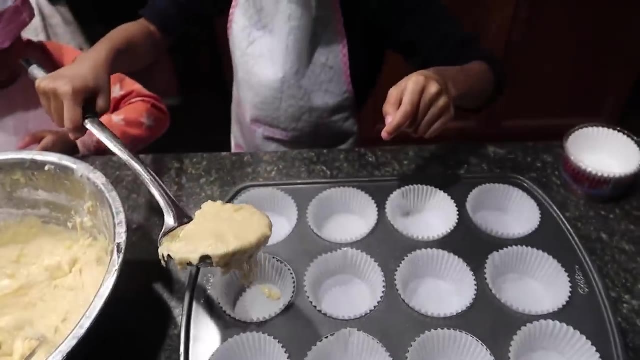 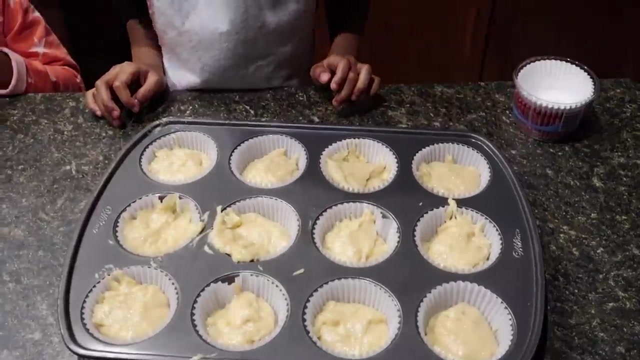 None, Okay, Now I'm gonna get these scooping, Scooping. Get this out, Get some of this in there. Ooh, sorry, sorry, sorry. Okay, we're ready to put in the oven. Let's call Daddy. Daddy, we're ready to put in the oven. 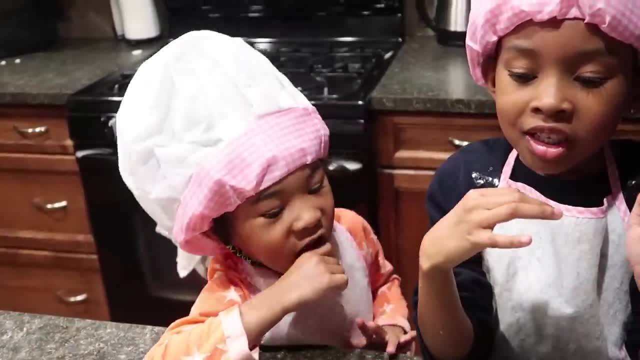 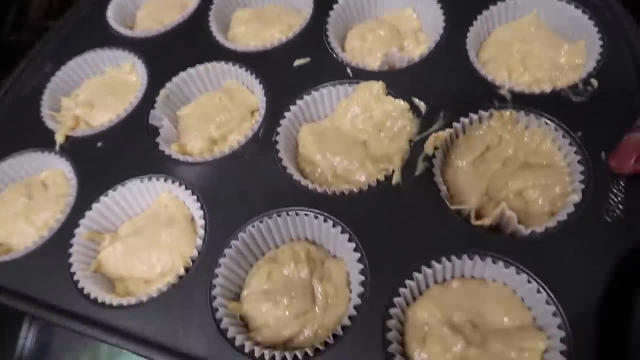 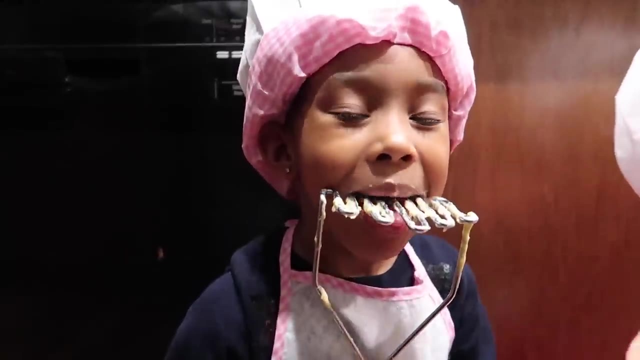 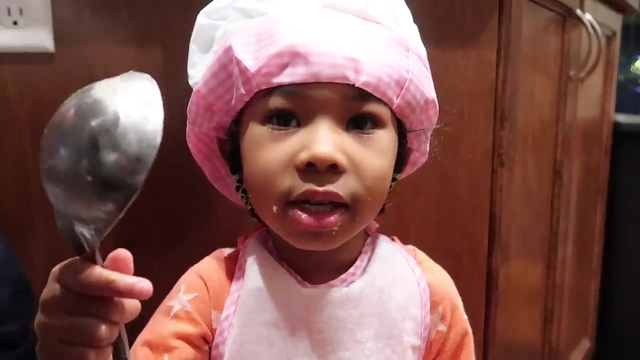 Okay, Daddy, we're ready to turn it up. and, Daddy, And now we wait. How long is this going to take? Daddy said about 15 minutes. Toy food, don't take this long. Yeah, because this is not toy food. 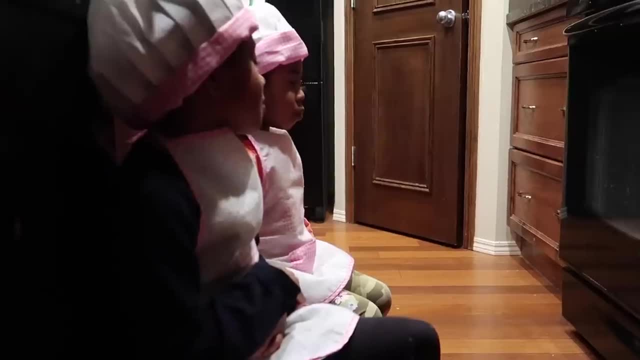 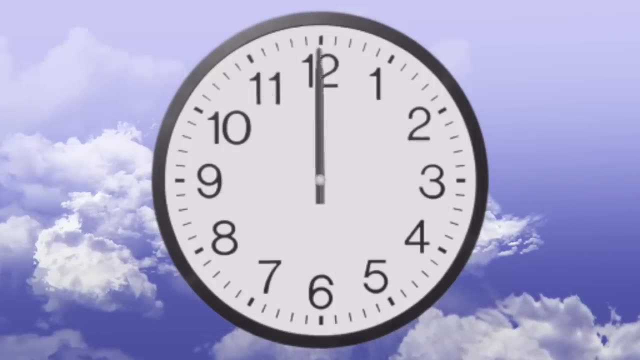 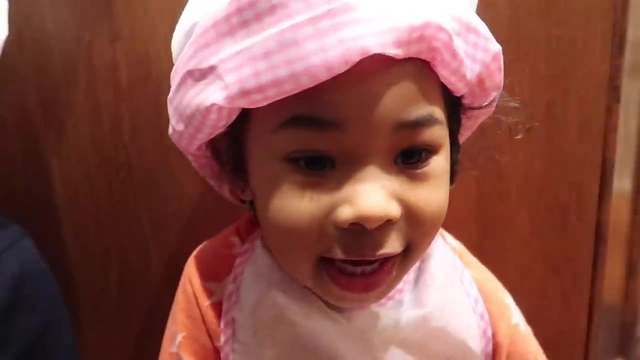 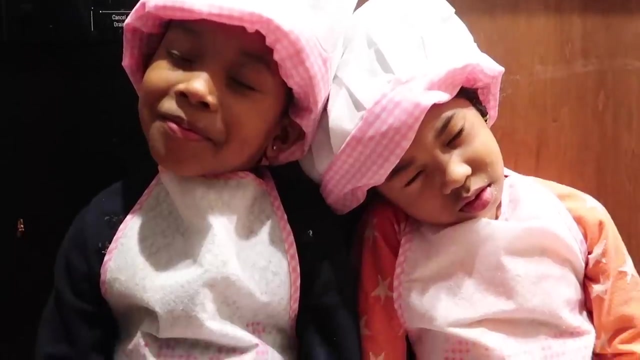 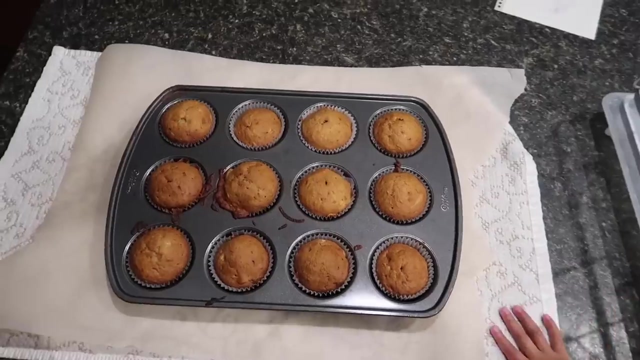 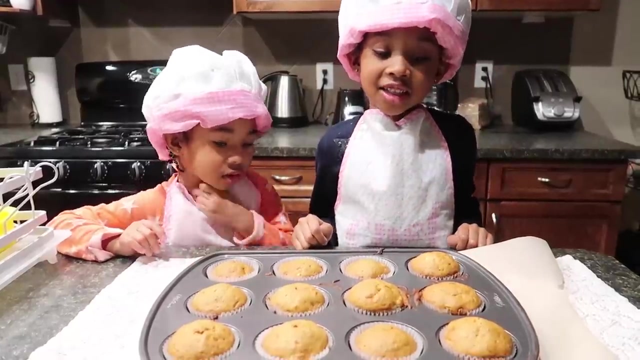 This is real food. At least we get to eat this. Ah, so boring. I'm thinking I'm going to take a look at that now. Yay, Oh, so fun. I can't wait to eat these, Me too. 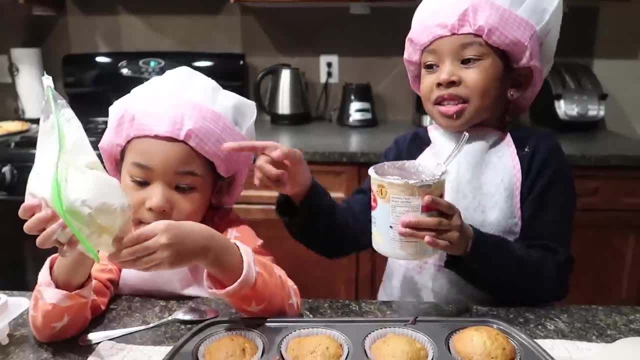 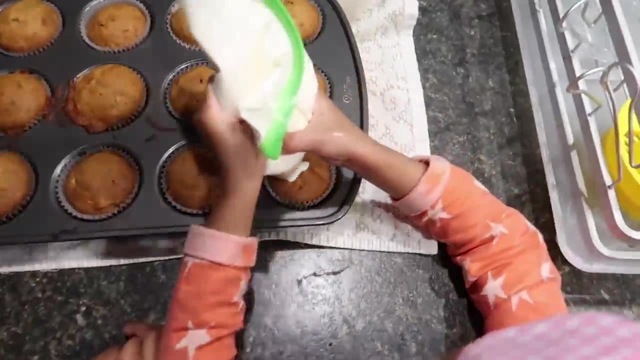 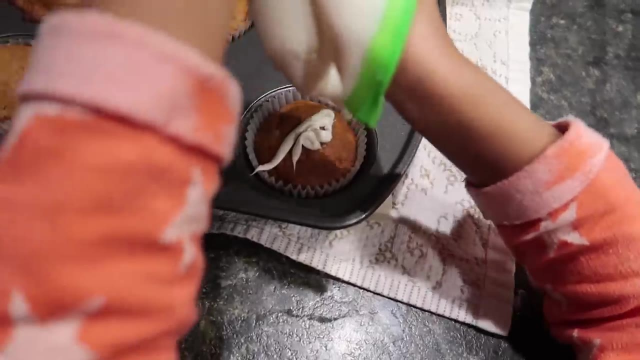 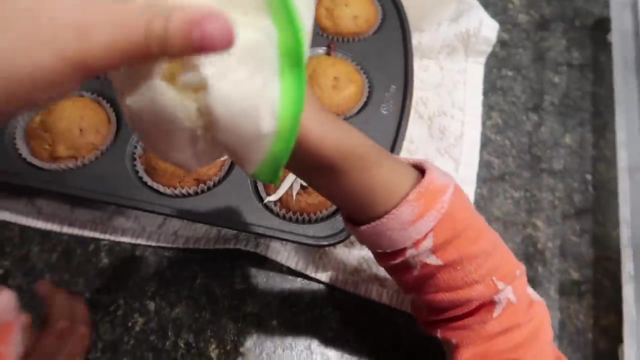 Oh, we can't forget the whipped cream. We put some in this bag so we can squeeze it on Squirt. I'm going to go first. Oh, that's so nasty. That's enough. Okay, my turn. All right, my turn. 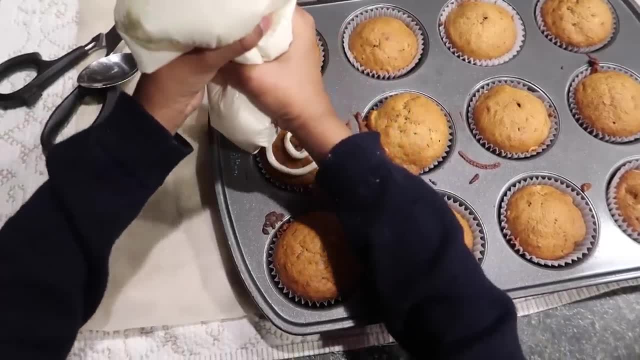 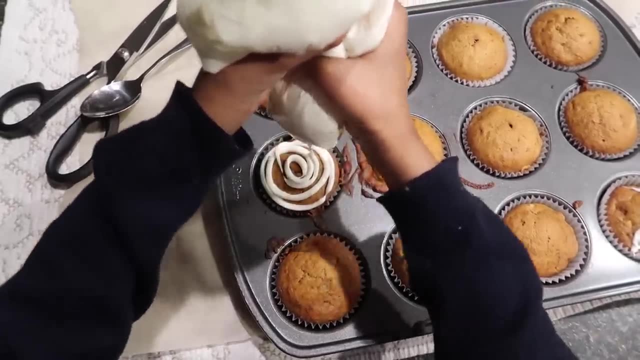 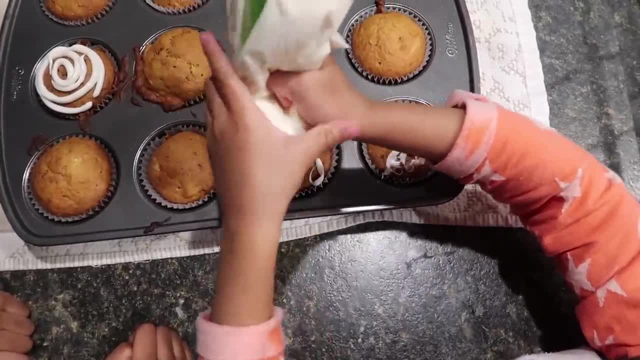 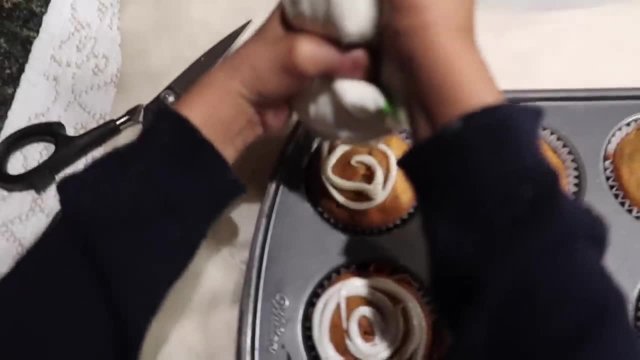 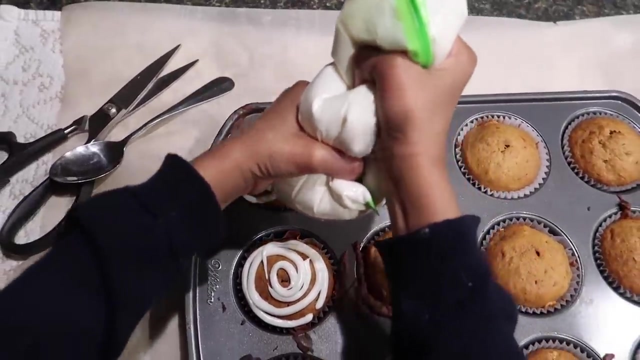 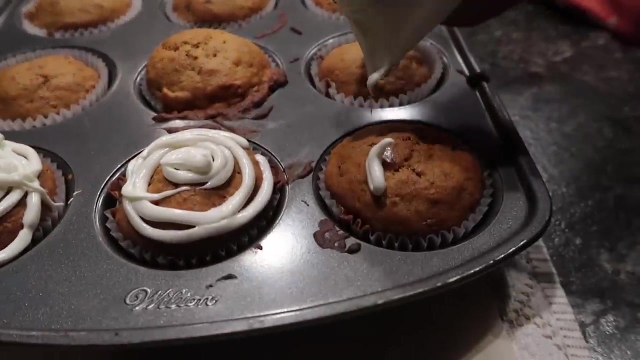 Swirly, Swirly, Baby, Baby, Baby. Right wing, That's better. Boooooo, Boooooo, The green is going. My brother did this one. You have to wipe real good Pop, oh you're. 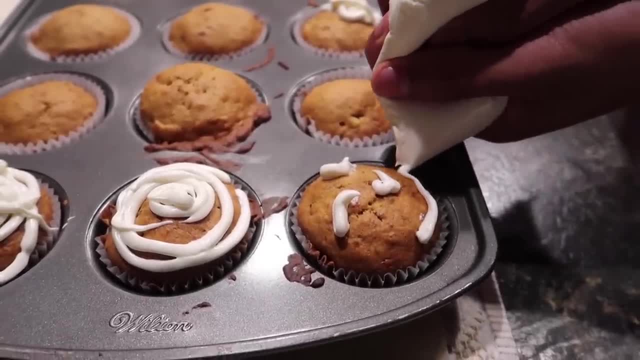 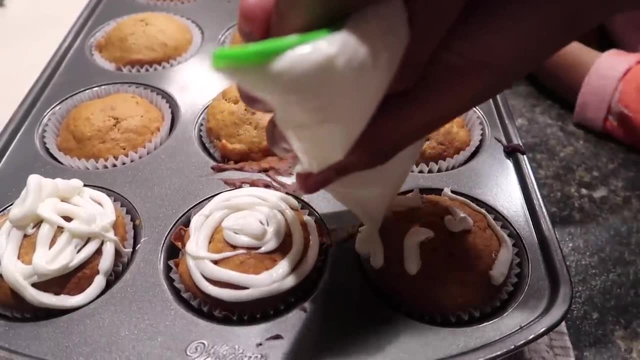 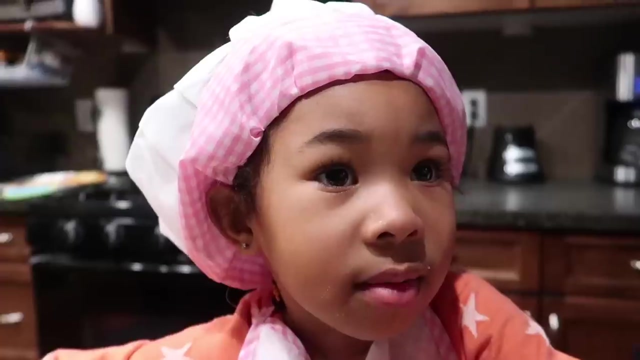 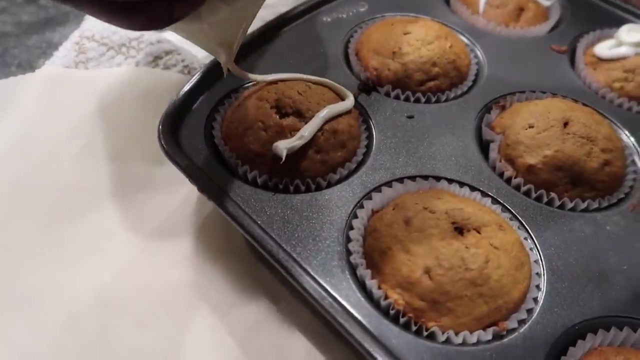 This looks like you're doing the. You're doing a face. Get some hair, Get some hair. It looks like a hat. It looks like Boooooo. My daddy did this one. What is daddy making? Daddy's making a D. 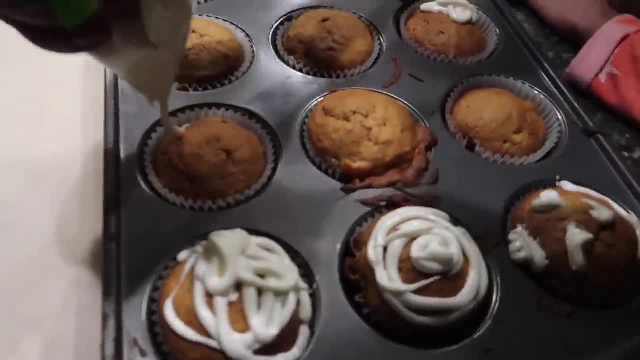 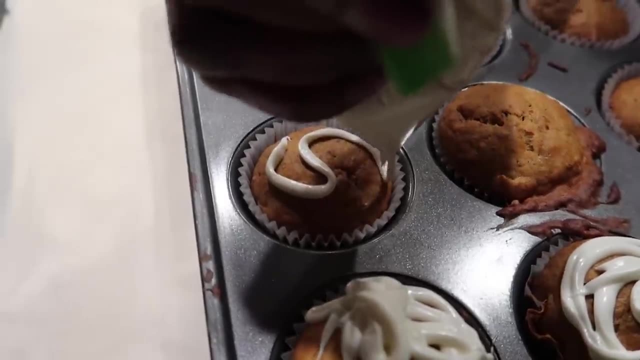 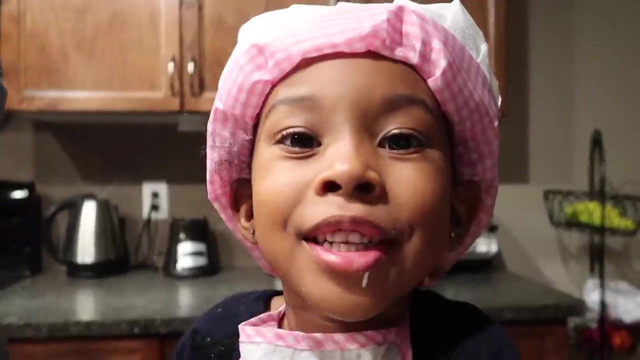 D for daddy. Daddy, somebody wants an O, That's an O. We could play tic-tac-toe. O, O, O, Daddy, the O doesn't work. Yep, you could do O. My mommy did this one. 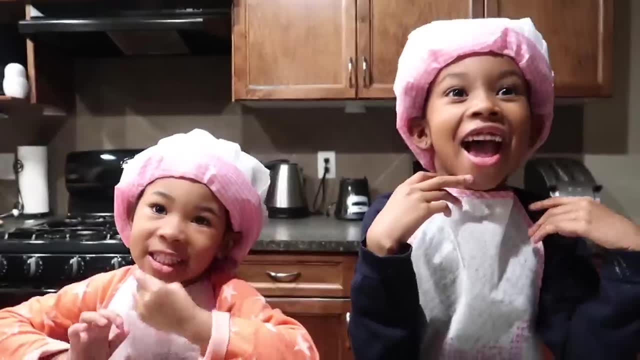 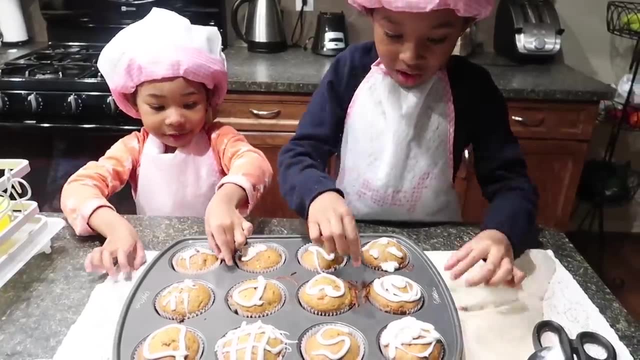 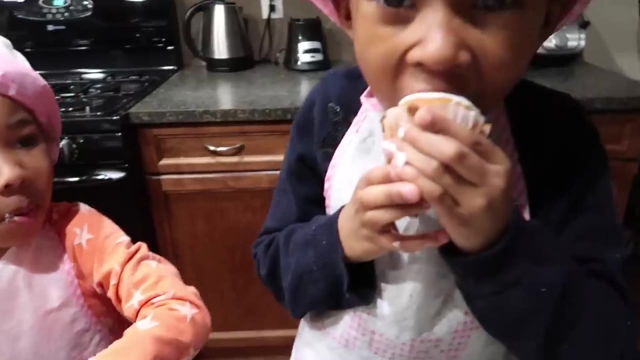 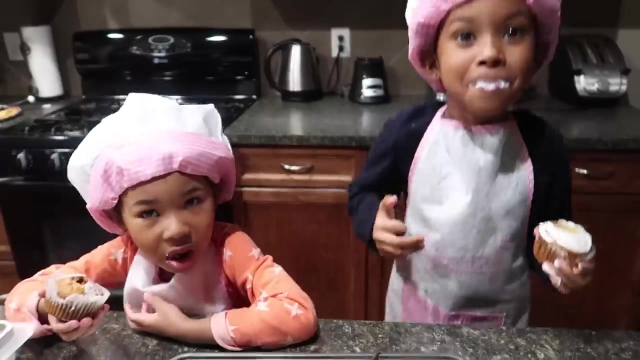 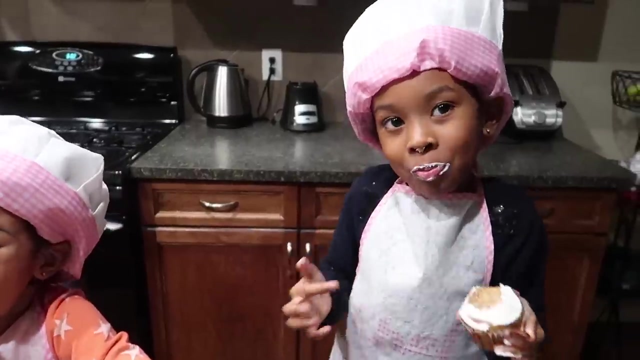